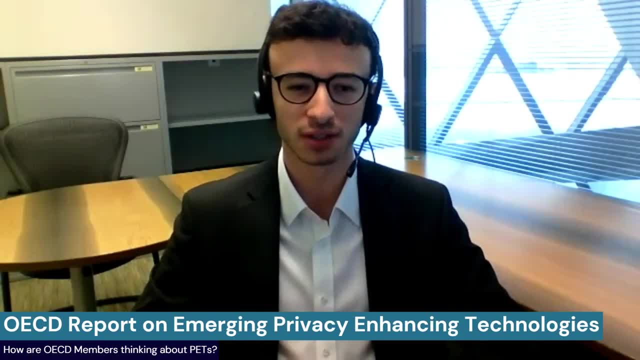 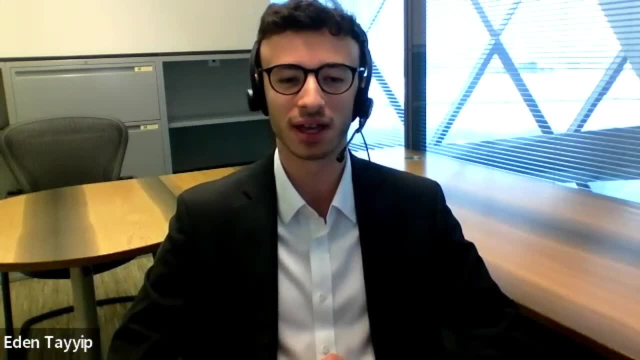 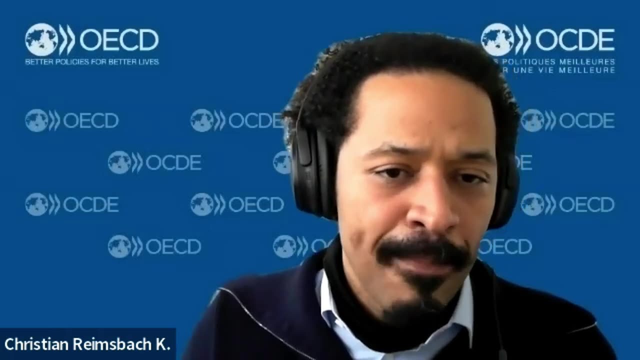 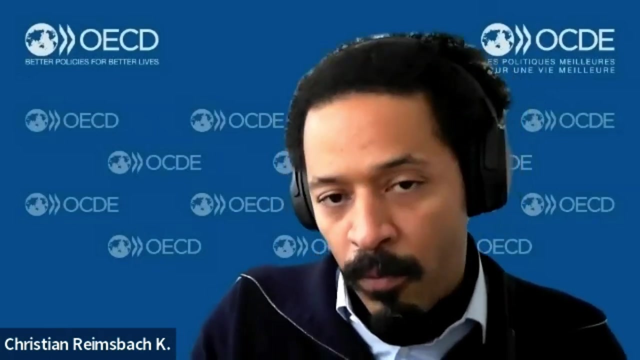 I understand that your report was informed by questionnaire to your member countries. How are your members thinking about pets? Are they welcoming these technologies? No, absolutely. I mean, I would definitely emphasize that what really makes this report unique is the direct contribution of our members and partner economies through the questionnaire. 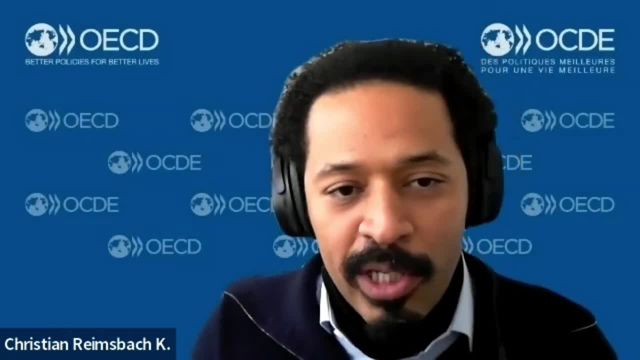 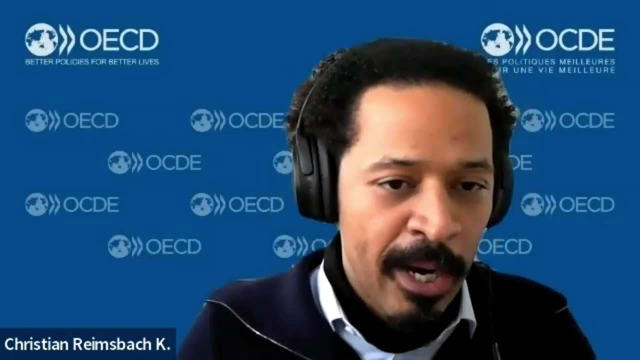 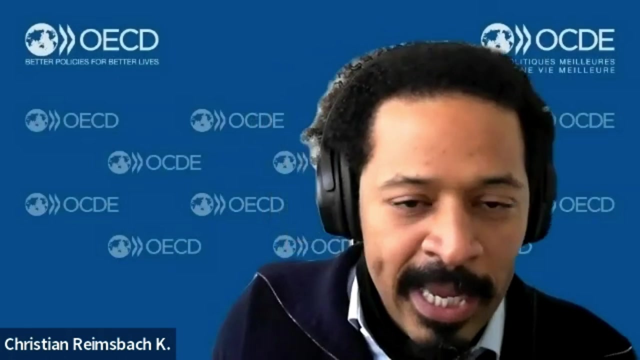 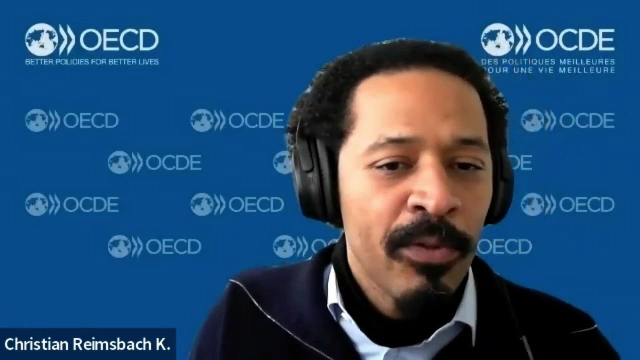 And I really would like to take this opportunity to thank all government agencies, all countries that have participated and responded to the questionnaire. So this is important. Number two, and I think this is an important caveat that I'm now about to say, only 22 countries responded to our questionnaire, And this is, if you know. 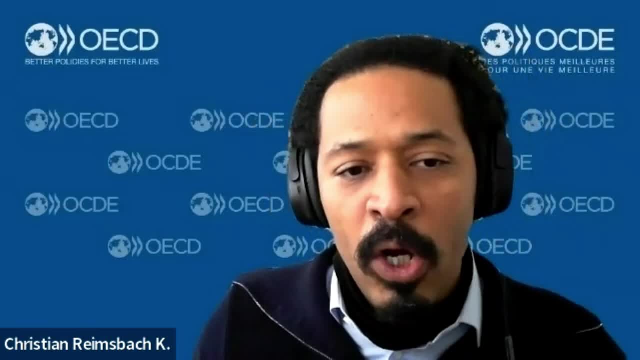 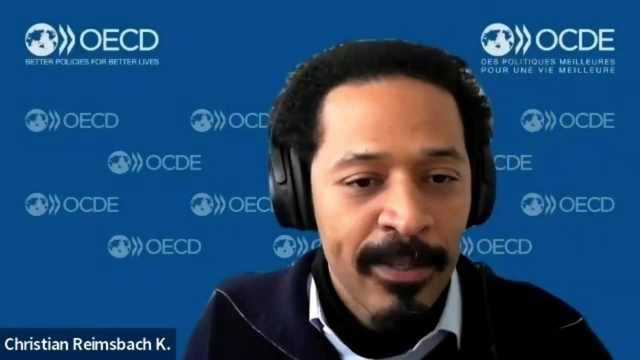 if you are familiar with the OECD, you know that this is a low response rate for OECD standards. Also, if you take into account that the OECD has 38 member countries. Now why am I emphasizing this? besides the fact that it's always good to know the 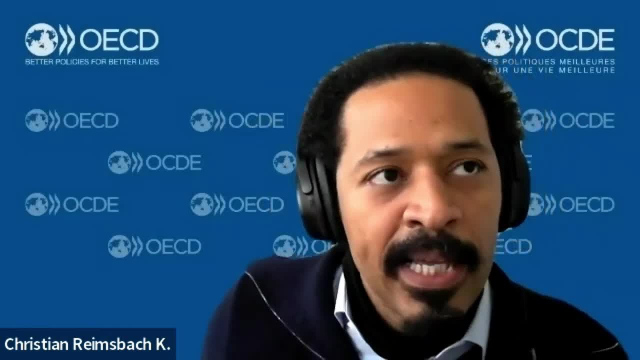 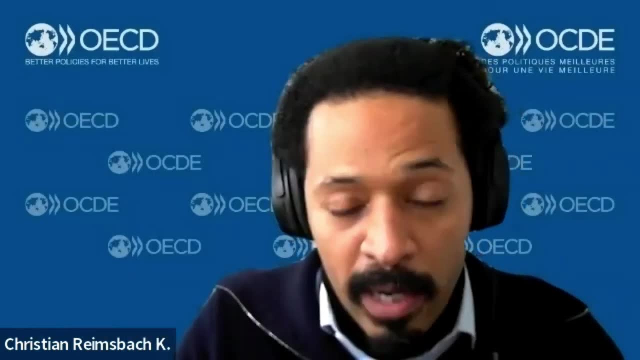 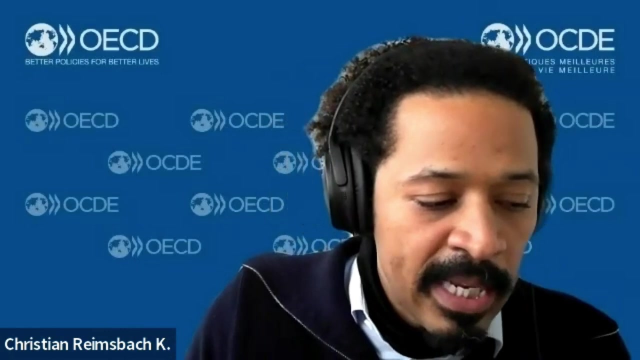 baseline, so to speak. The reason why I'm emphasizing this is because, while thinking about the reason of this low- and there may obviously be a lot of different reasons for the low response rate- I think to some extent you could make the argument that it also reflects the fact that a number of countries are still not sure. 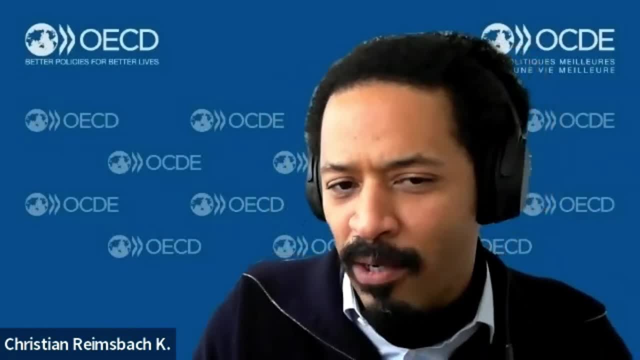 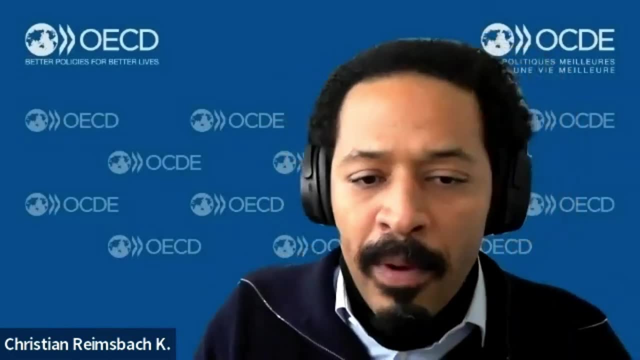 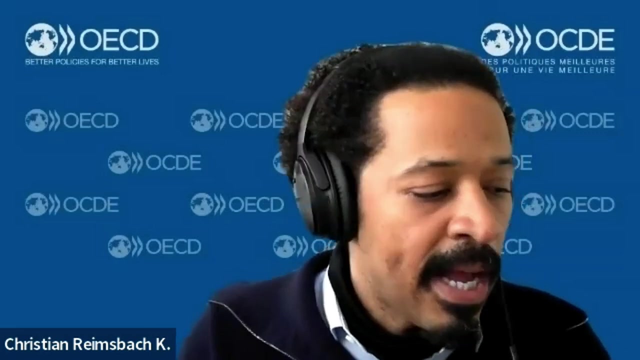 what exactly to think about privacy enhancing technology. So it's a in particular, when it comes to the emerging privacy enhancing technology, I think there is still a number of countries are still starting the not starting, but I would say thinking and. 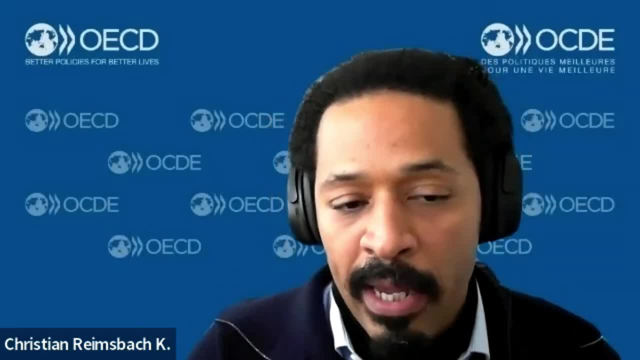 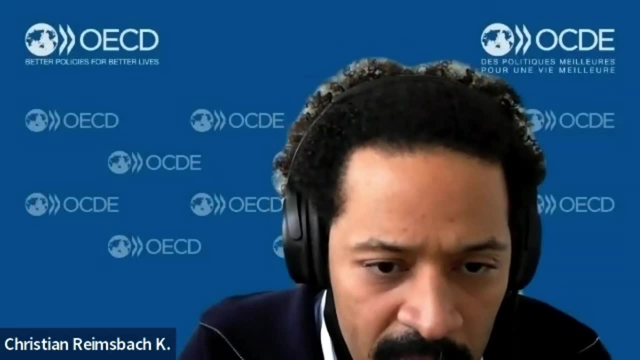 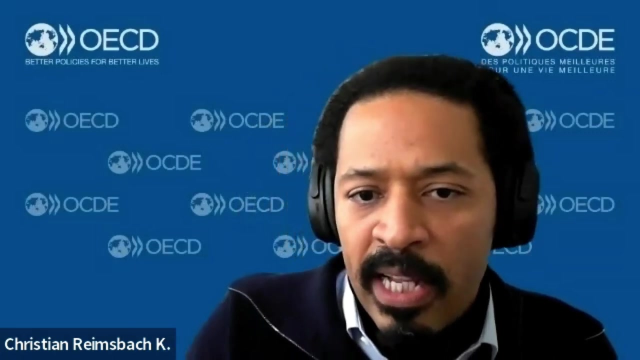 considering what it means exactly for the data governance and privacy frameworks and the policies. So this is number one. number two: So concretely, what in terms of what countries are doing? I mean, we noted two important things. One: we noted that countries have clearly recognized 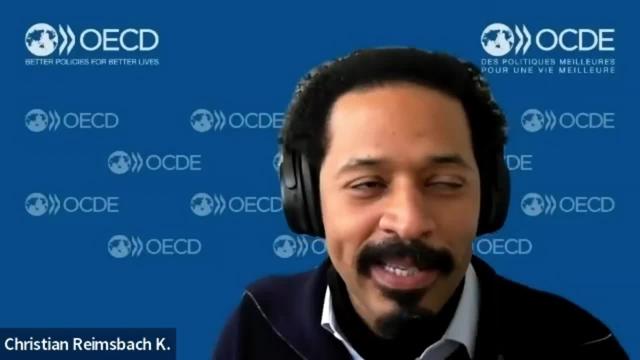 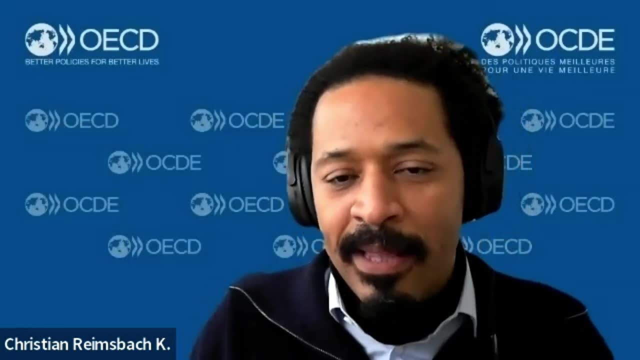 or more or less clearly- I think that's an important point too that we may discuss later on- have recognized at least that pets are recognized in privacy and data protection frameworks, And the reason why I was hesitating about clearly is because in many instances,